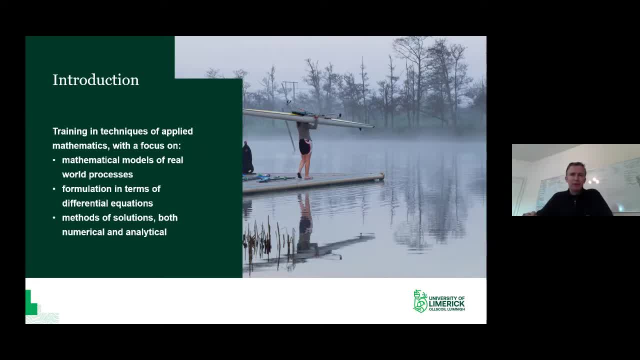 Very important is the formulation and structure In terms of differential equations. so if you know your applied mathematics background- and I hope those of you interested in this course would have seen differential equations and other applied mathematical techniques before- you'll know that differential equations are the way that we use to take models and take rules for how things change in time and to turn those into predictions for what will happen in the future. 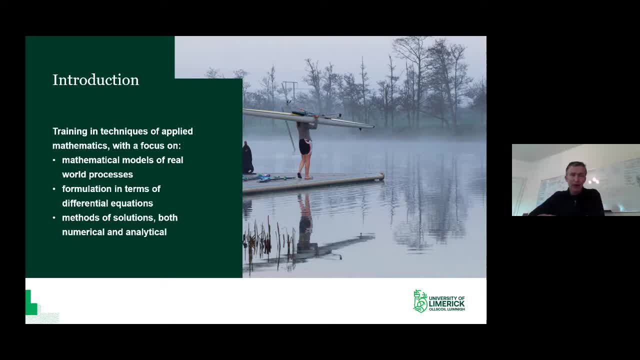 So I'll give you some examples of that too in a few moments. And, very importantly, parts of modelling are both the development of models- so taking a real world problem- and turning it into mathematical equations. but then of course we need to be able to solve those equations too. 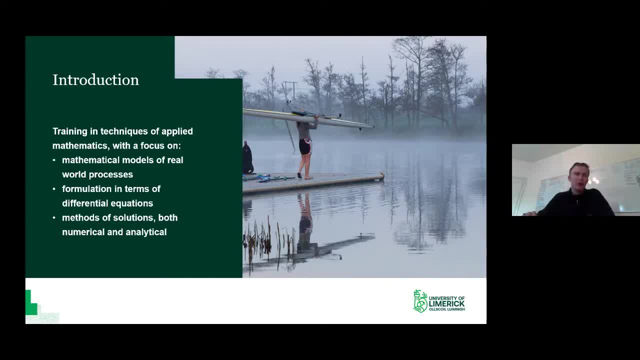 So the methods of solution, which are we tend to break into analytical methods- things that you can do with pencil and paper, and numerical methods, where you need to do computer work, are both very important parts of Masters in Mathematical Modelling that we'll be teaching you here. 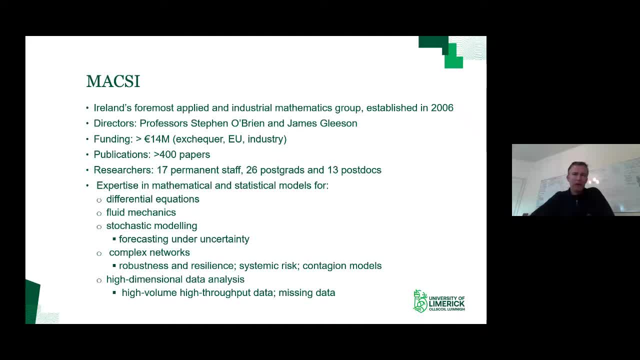 So I'm a course co-director of a group called MACSI, which is the research group within the Mathematics and Statistics department here at the University of Limerick. We're one of the top groups in the country, perhaps the top applied mathematics group in the country. 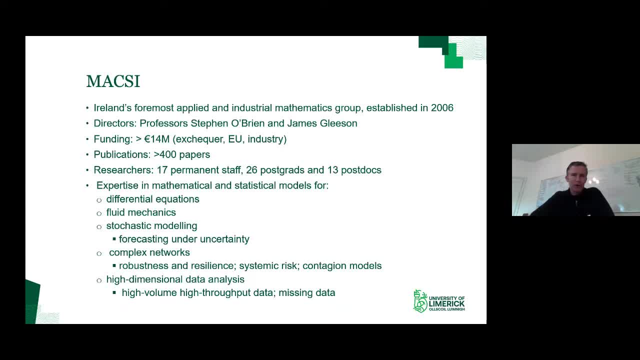 We've been very successful over the years in gathering competitive funding in writing papers, and our areas of expertise cover a wide range of mathematical and statistical techniques, As I mentioned: differential equations, fluid mechanics, modelling under uncertainty- my own area of complex networks- and contagion modelling. 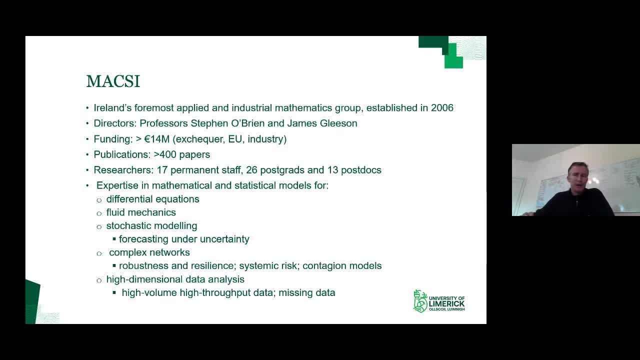 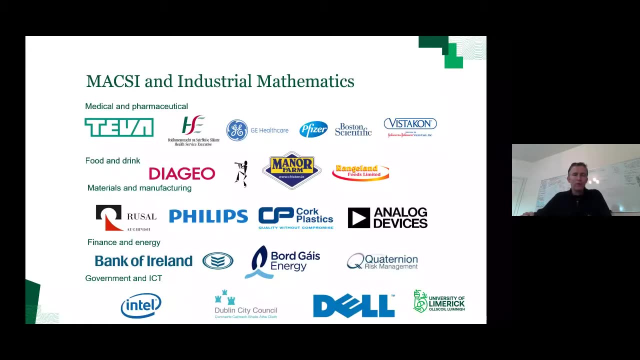 and more and more recently I focus on data analytics and data analysis, which is a very important part of our statistics group and links up with the mathematical modelling as well. We do mathematical modelling in the real world. That's a very important focus of both the MACSI group in general. 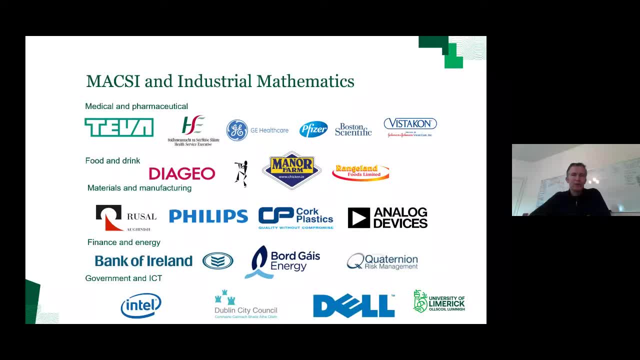 and of this Masters in particular. So it's not just applied mathematics to prove theorems or to know a little bit more about mathematics. We very much focus on applying and solving real world problems. So this slide just gives you some examples of the companies that we've worked with. 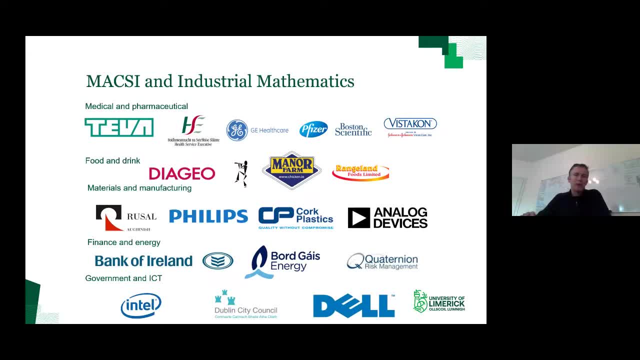 over the years, because mathematical modelling deals with the world where there are real world problems, And much of mathematical modelling is about taking a real problem, a problem that someone has in industry or someone has in the scientific realm, and turning that into equations. 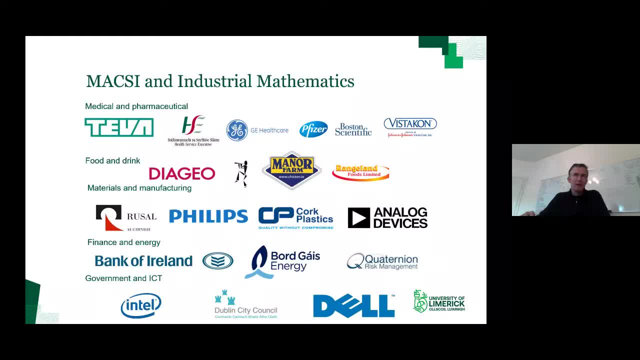 That's a non-trivial part of the step. It's something that you can know a lot about solving mathematical equations and still not know anything about how to turn a real world problem into mathematics. So that first step is an important factor. That's the focus of our Masters. 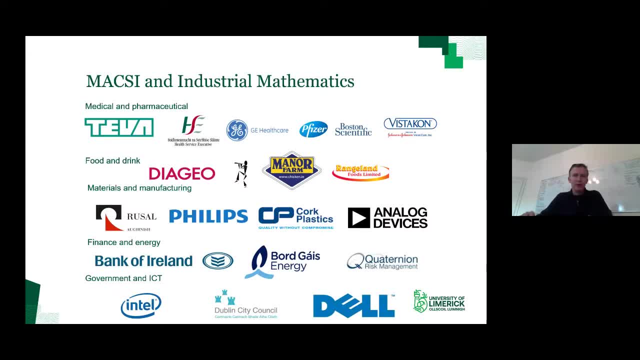 Although of course, you also have to learn the techniques for solving all the equations as well, and that's an important part. Another important part- and I'll show you a little bit more about this in a second- is being able to explain the results back to the stakeholders. 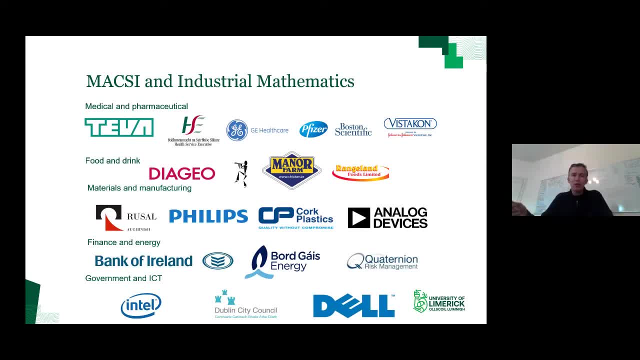 back to the people again, be they in industry or be they in science, who need to know what the results mean. So I'll talk a little bit about modelling of COVID-19 in a few minutes. I'm involved in the National Modelling Advisory Group that works with NPHET. 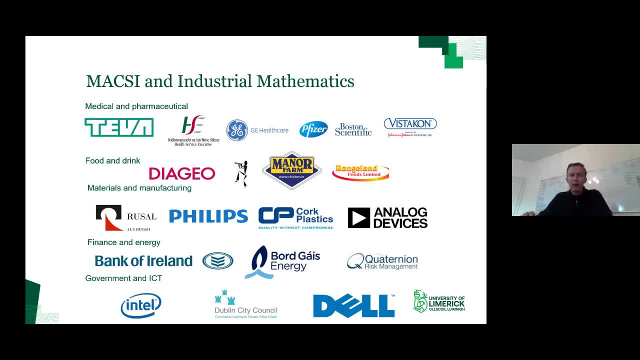 who's the National Public Health Emergency Team here in Ireland. So at the government level we're giving advice on policy making, and a lot of that policy making, or a lot of the advice we give, is based on mathematical models of the type that I'll show you. 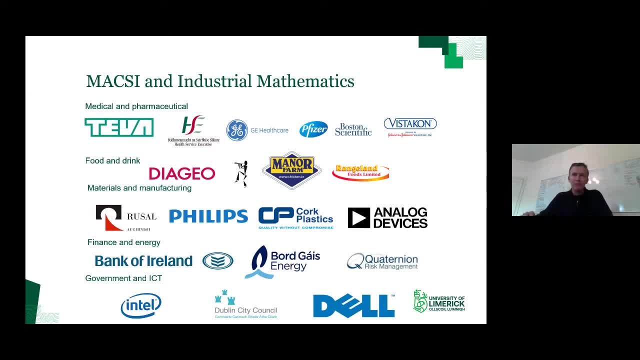 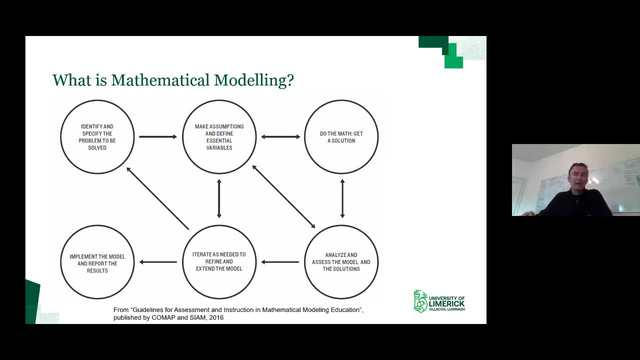 and which are based on the kinds of ideas that we develop here in this Masters. So mathematical modelling as an overall academic exercise, if you like, has multiple steps, As I said to you before. there's the bit where you do the mathematics. 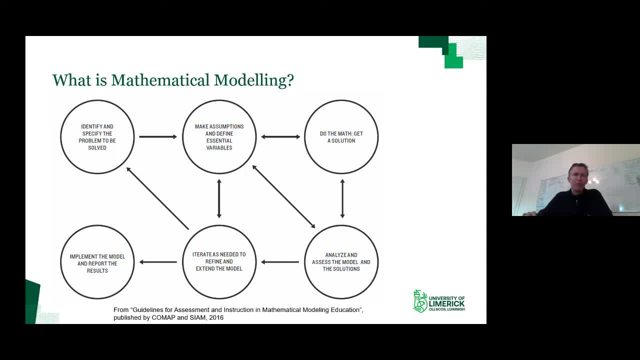 for a set of equations and get a solution. But before that it's important that we identify and specify the problem to be solved. So again, talk to someone in industry who may have a rather underdeveloped view of what exactly the problem is. 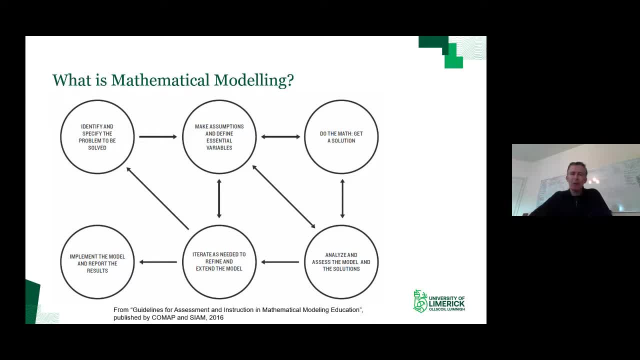 They know they have a big pile of data, They know they have a specific problem on the production line, but they don't have a mathematical language to explain that. So the job of a mathematical modeler is to help turn that problem into a mathematical one. 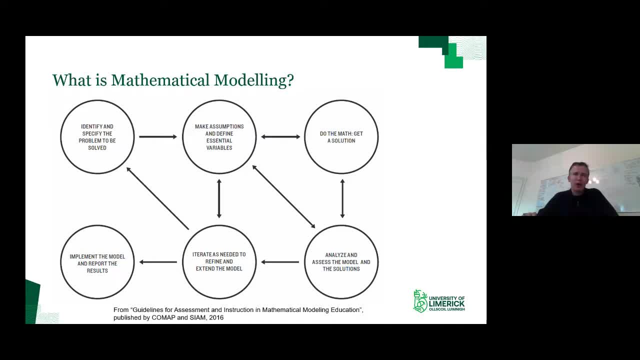 So, making some assumptions, define what the essential variables are. then take that perhaps very simple model. initially, do some mathematics, find out what the solution of the equations that you've written down are, and then the very important step of comparing that back to the real world. 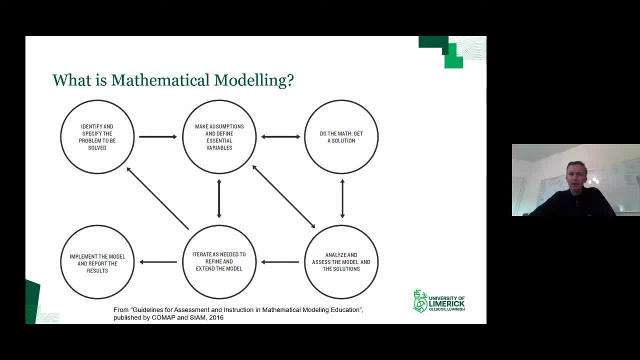 So if you said something about how the production line should change, or you've said something about the number of infections that may happen in COVID-19,, for example, we need to compare that back to what happens in the real world, And all models are imperfect. 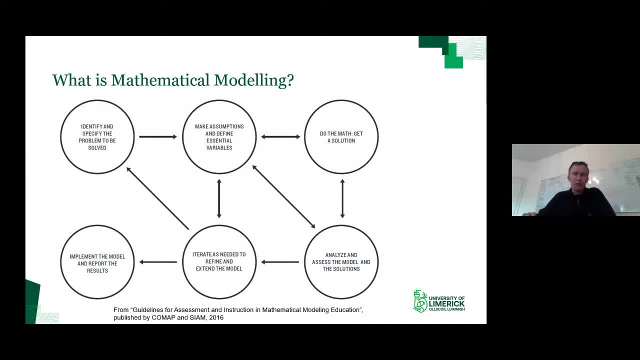 Much of the skill in modelling is in understanding what assumptions are vital and what assumptions can be changed, and why you would need to do that based on how well your model compares to reality. So modelling is really an iterative process. It's a process where we go around in a cycle. 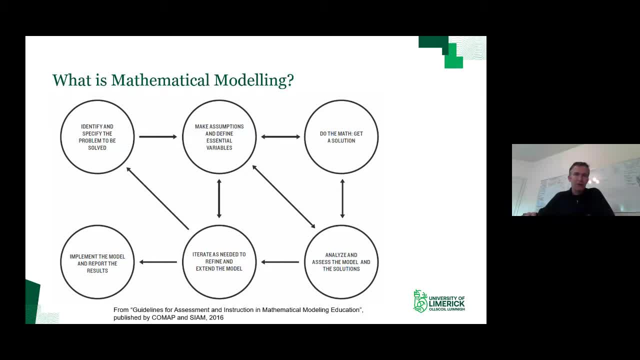 We continually improve the models, compare them, solve them, check them back with reality. And as the models get more complex, of course it gets more complicated to solve the models and to get comparisons with reality, But always, in the end, the focus is on reporting back to the real world. 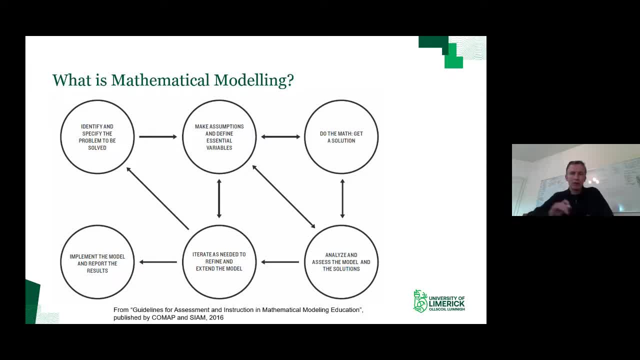 and connecting back to the real world. So again to industry or whoever has set the real world problem in the first instance. So an important part of modelling is that collaborative and communication part, where you're able to talk to people who are not mathematicians. 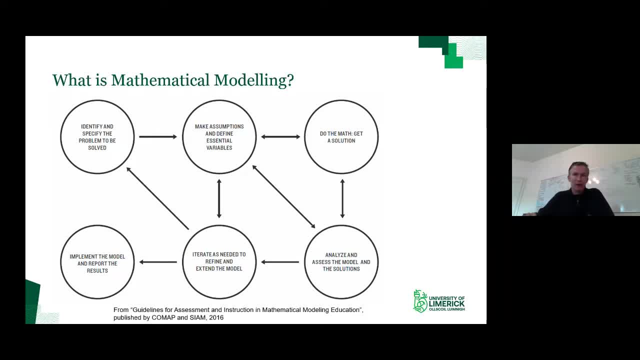 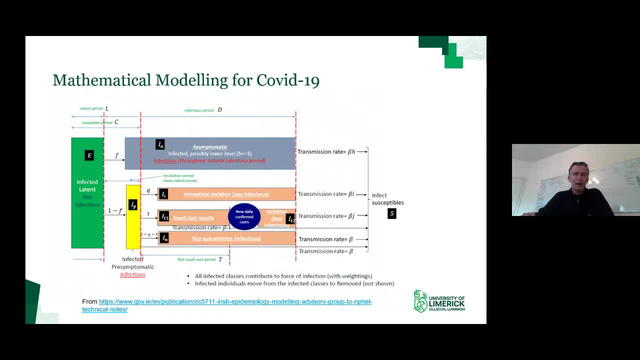 and able to explain results that come out in mathematical language, translating it back to the language of the real world scenario. So I thought I'd give you a quick view of some of the things that we're doing on that national COVID-19 modelling group. 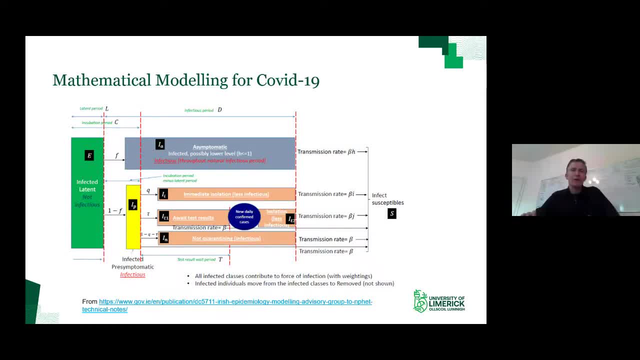 just to give a flavour for how all these things pull together in terms of a very obviously important and urgent real world problem. The slide referenced down the bottom is to the technical notes that we've released on the Department of Health website, So there's further detail there if you are interested in these models. 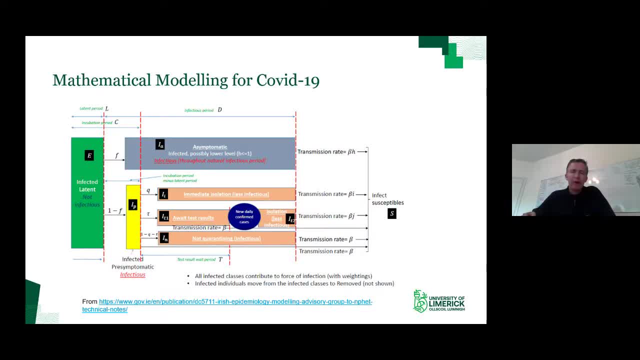 But essentially the model. one of the models that we're using for COVID-19 is what's called a compartmental model, So people who are infected with COVID-19: in the early days of their infection they have the virus in them, but it's late. 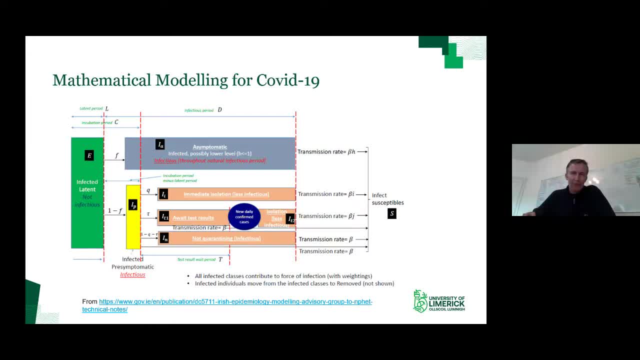 and they're not infectious for three to four days. Then there's a short period of one to two days during which people are not yet showing symptoms. So the point at which people show symptoms is this red line here, But before they show symptoms, people are infectious. 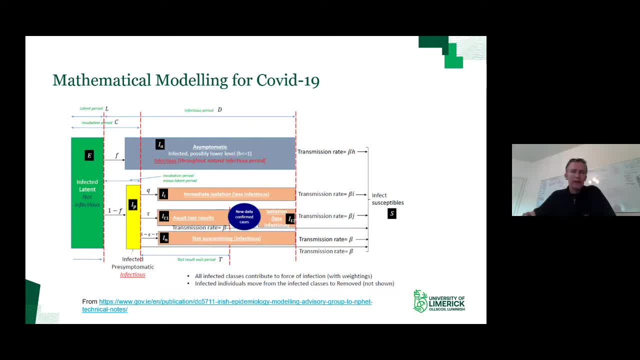 And all this work is based on extensive literature reviews by a biological parameters team also part of the modelling group. So they've looked at all the details in the emerging scientific papers on COVID-19 to understand the details of how the virus works, And one of our jobs is to turn that into a mathematical model. 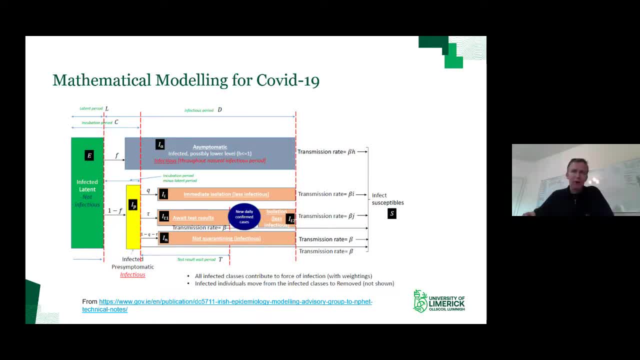 into a picture like this and then into a set of equations to help predict what will happen in the future. So before people become symptomatic for one or two days, they are still infectious and can infect other people. And then, even when people show, 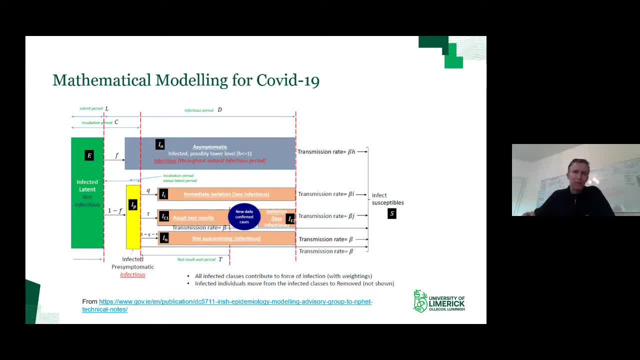 some people show symptoms. So this group of compartments here include all the people who show symptoms. They go to be tested, or perhaps they self-isolate, or perhaps they do neither of those two things, And there's a significant cohort in COVID-19 who don't show symptoms. 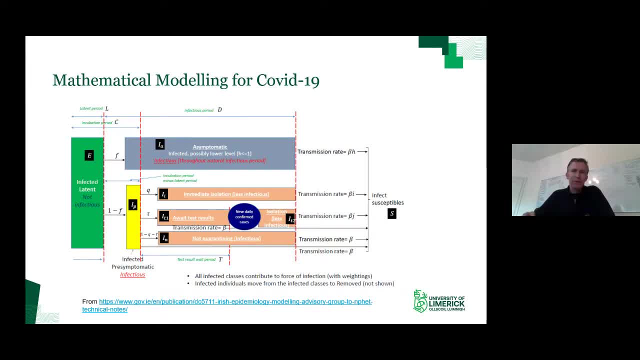 but still are infectious. So that's what's called the asymptomatic infected people. So this is a. in mathematical language this is called an SEIR model. S stands for susceptible, The E stands for exposed. I is the infected people and or the recovered. 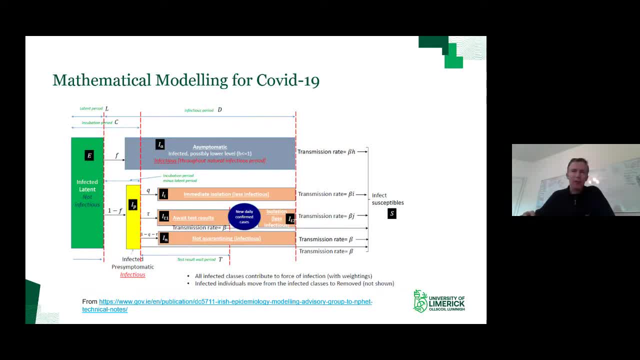 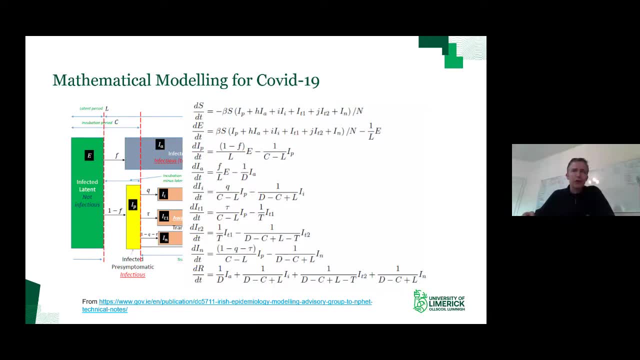 And how the people move through these compartments is driven by differential equations. So this is a set of differential equations that describe the model I've shown you in pictures here, Rather complicated. there are a lot of parameters in here. but, as I said, 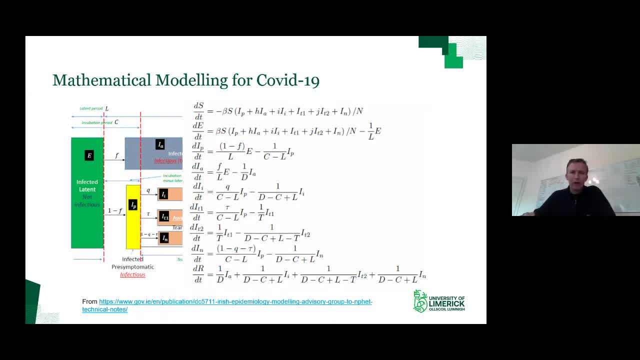 part of the mathematical modeling process has been working with our colleagues in biology to understand what those parameters are and what they mean in terms of the mathematical model, Turning those into equations and then, once we have equations, we can use that to compare with data from the past. 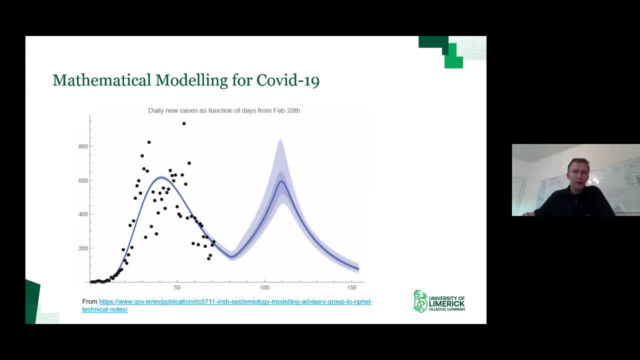 So obviously working with our statistical colleagues is an important part of this modeling process as well. So these data here show the daily confirmed new cases for COVID-19 from February 28th- first case in Ireland up to just early last week, And you can see: 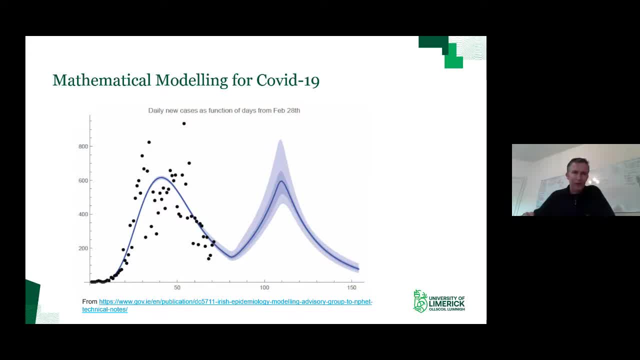 the trend of the cases went up and now, thankfully, has been coming down And we've been working on what might happen in the future. So mathematical modeling allows us first of all to get a good fit of the equations to the data that we've seen so far. 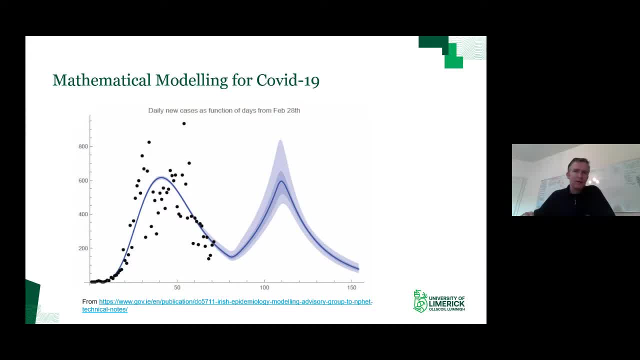 but, more importantly, it allows us to think about what might happen in the future. So this was the date where lockdown was lifted last Monday. so this was done a little bit earlier this Monday, And what we hope will happen is this: that the infections will continue. 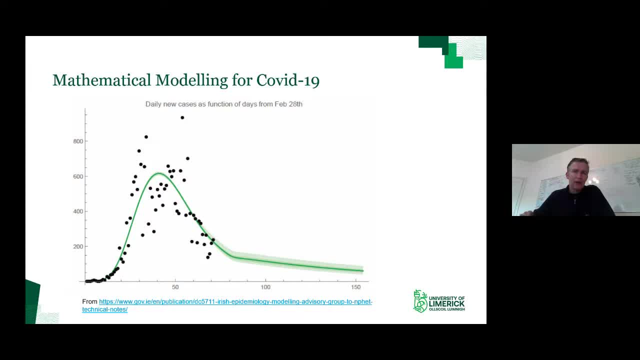 to die out and decrease, But depending on how mixing in social contacts happen, we could be in a case like this where we get a second peak, And one of our jobs right now in the modeling committee is to watch the behavior of these curves and these data points. 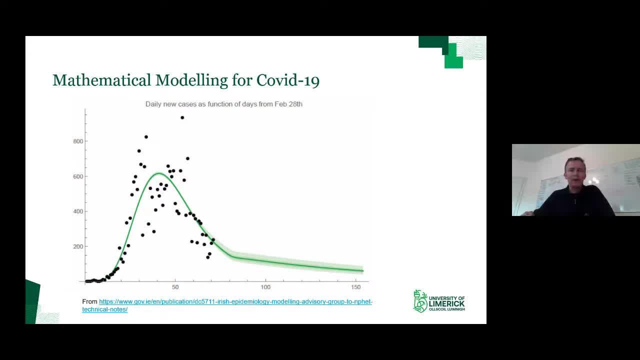 as they come in. very noisy, as you can see, but still fitable with models like these to try and ascertain early enough which of these types of scenarios might happen in the future. So that's just an example, I guess, and I thought a very topical example. 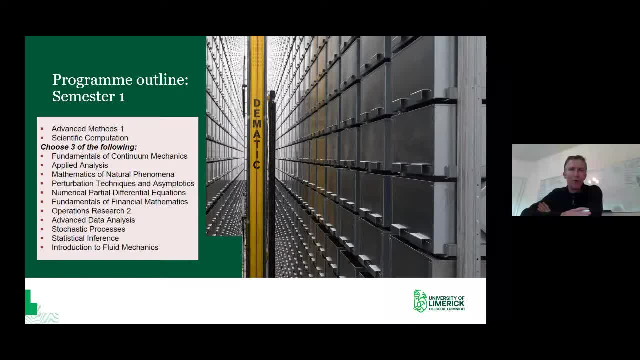 of how mathematical modeling is used to solve some important real world problems. Let's go back to the masters and talk about how you might learn the techniques to get involved in modeling like that- The courses that taught masters program. that means it runs over 12 months. 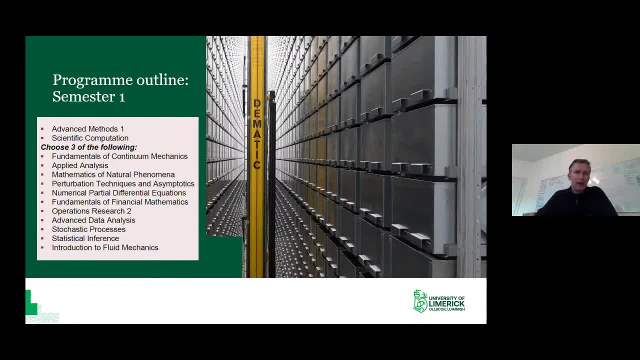 Semester one starts in September And in this course you'll take five modules in each semester. So here there are two core modules- advanced methods one and scientific computation, And they essentially respectively teach you about solving mathematical equations analytically and solving them numerically. 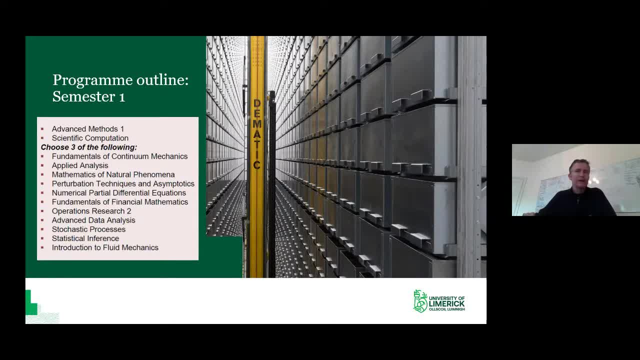 So we need to make sure at the start of this program that you have the mathematical techniques that you need to be able to develop models and help solve those, And then, in addition, you can choose three electives out of a fairly large set of choices here. 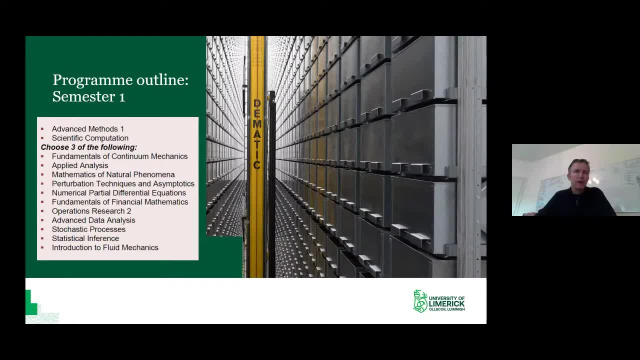 And those choices include statistical modules, stochastic processes and statistical inference, for example, Data analysis, Or they include some financial math modules, if you're interested in financial mathematics, Or classic applied math modules like fluid mechanics and continuum mechanics as well. So there's a set of choices. 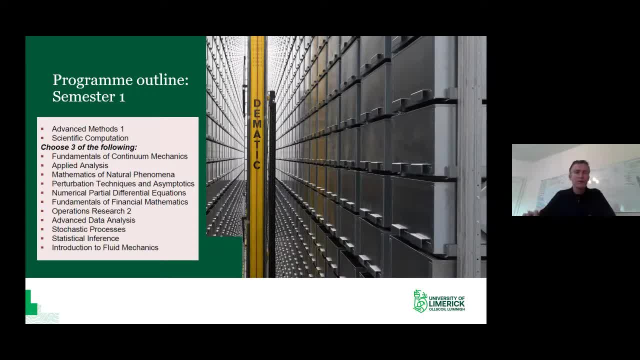 and when you might arrive in UL. before we start semester one, as part of the induction day, we'll sit with people and explain what each of these modules is about and how that might fit into how you'd see this masters working for you in terms of where you want to go next. 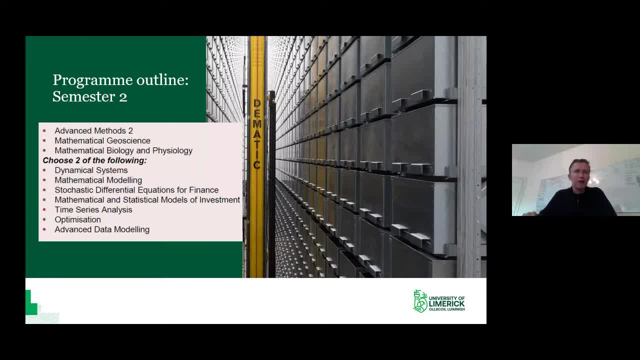 In semester two, there are three core modules, One of which is the mathematics courses, and then some applications courses, including ones around biology and modeling of that type, And two electives, again with the electives allowing you to go down a route of data or statistical analysis. 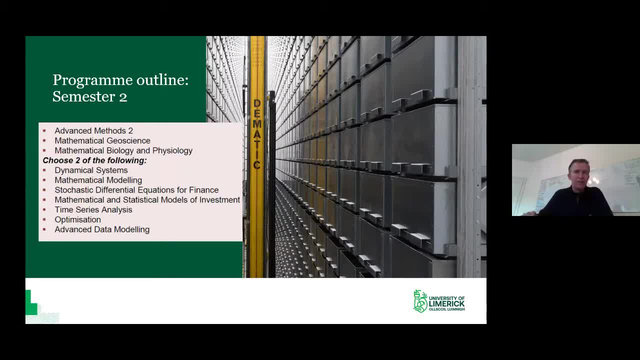 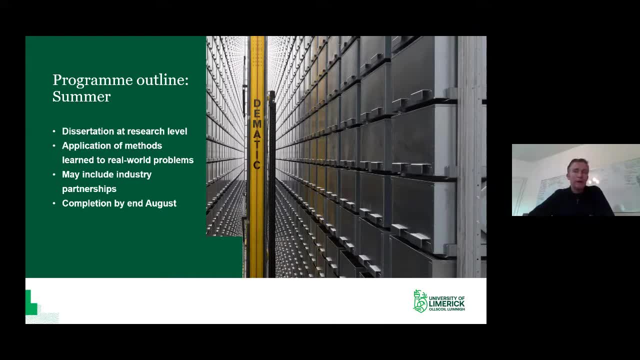 to do a classic mathematical modeling or to look at financial mathematics, which are the three main areas I guess that we see people falling into. That takes us to about May of next year and then the entire summer. for the summer you work on a dissertation. This is an important part of the program. 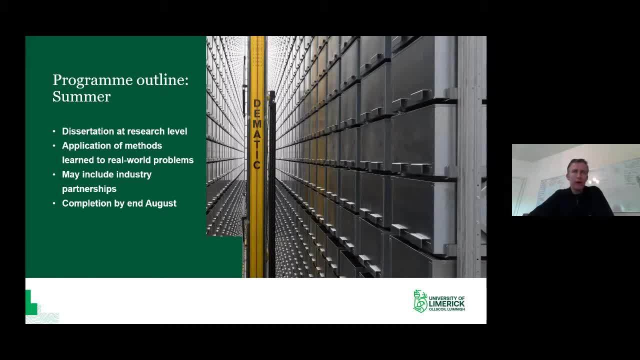 it's 30 credits. that's one third of the program in full. so it's not a minor part of the program, it's a fully incorporated part of it and it should be at research level. so you'll be supervised by someone who's doing research work. 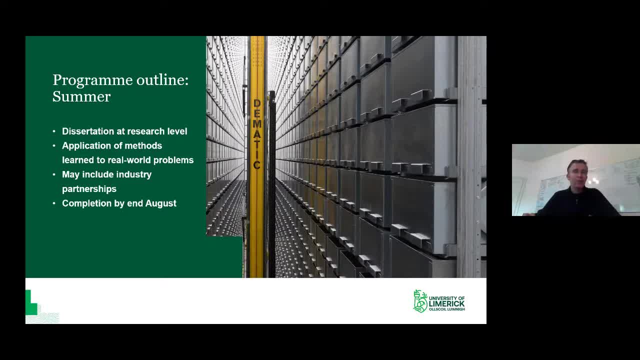 and these dissertations typically involve taking some contained part of that research work and working on it as part of your masters thesis. I'll show you some examples of recent dissertation topics that people have been looking at. It'll be as you've seen. the main focus is application to real world problems. 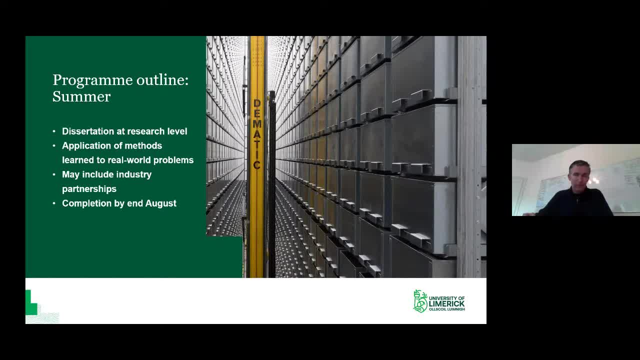 it'll include mathematical solution methods. it may include work with industry partners- for example, those real world problems may be motivated by work with our industry partners- and it'll be finished by the end of August or very early September. so essentially the entire program runs for about 12 months. 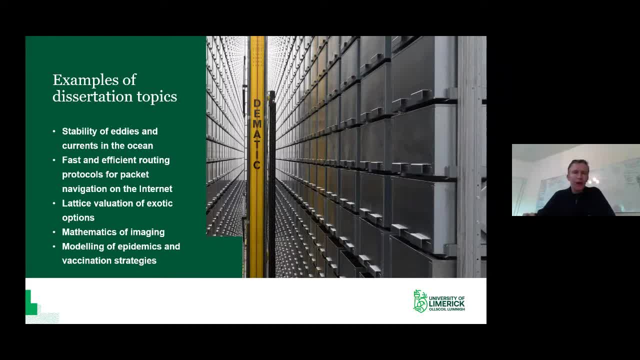 Just some examples of recent dissertations. again, mathematical modeling. it's a wide ranging topic because essentially what you're doing is learning to speak a language. the language of mathematics can be used to describe many different areas and applications, ranging, for example, from fluid mechanics at the climate and 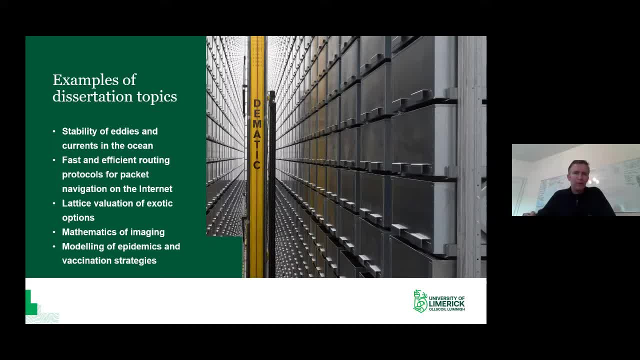 global level to the routing of packets on the internet. so motion to flow through networks, through financial mathematics. so evaluation of exotic options is a question of evaluation of financial derivatives. the mathematics of imaging is looking at x-raying, radar and other other mathematical, other techniques that are 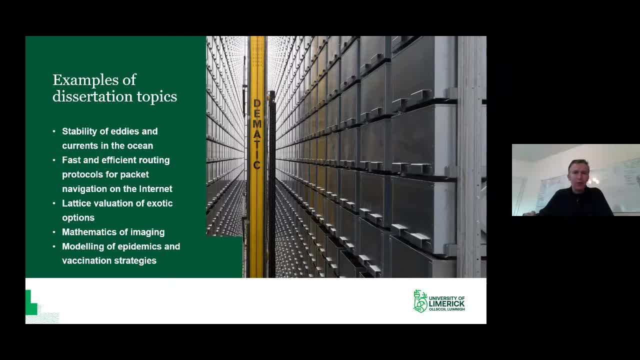 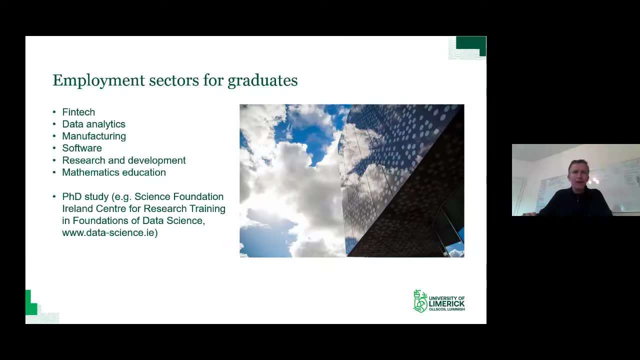 used to construct images either of bodies or of the earth. and finally, as you've already seen, modeling of epidemics and important topics like vaccination strategies, which I'm sure will still be on the agenda in this September. I'll finish just by giving you a quick view of the 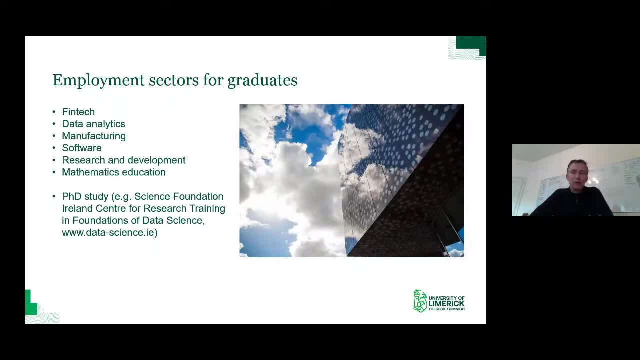 employment sectors that our graduates go into. graduates from this program have been very successful in employment. essentially, employers understand that having done this course we have that the graduates emerge with a strong ability to think, to apply mathematical and logical thinking to real world problems. some graduates will go. 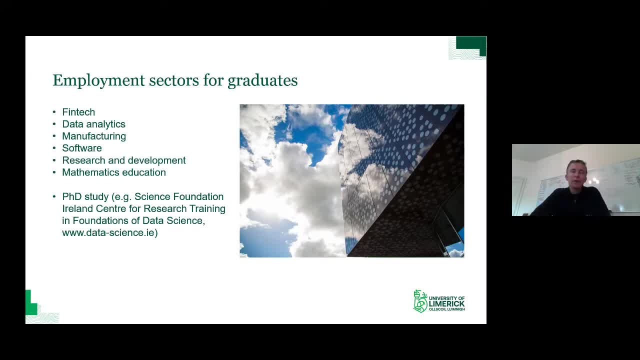 and not necessarily use advanced mathematical techniques, but they will be involved in jobs where they're using logical thinking and, I suppose, the ability to learn and to solve complicated problems, which is always something that's valued by employers. across many sectors, we've had a strong set of a strong 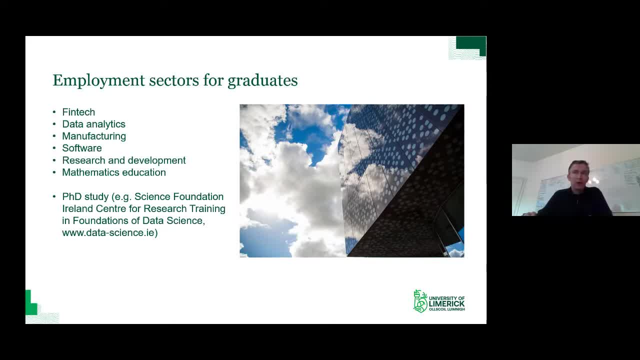 link for our graduates with fintech in general. so financial services, investment bank, evaluation of options- those are high value areas which have always taken graduates from mathematics and mathematical modeling. in recent years, data analytics has been a huge growth area and very many of our graduates have gone in that direction. 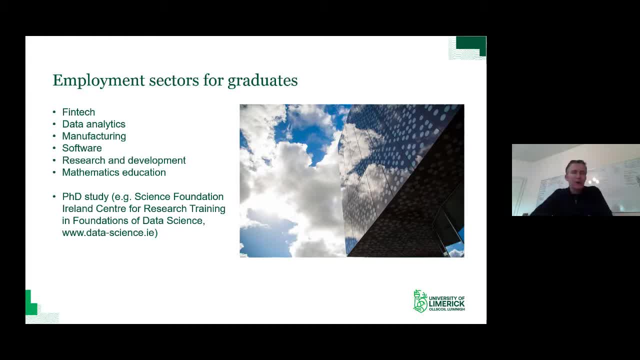 the manufacturing field again. sometimes people are surprised, but there's a lot of mathematical modeling, both in the engineering and on the data analysis side, and quality control in manufacturing. similarly, in software, the development of the ability to think logically through a problem and all the steps that are needed is a crucial 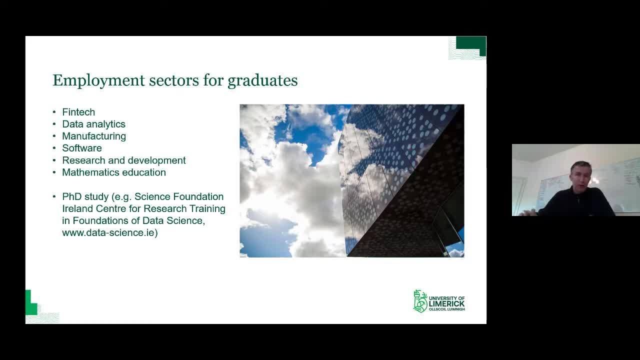 part to developing good software. people going to research and development. that's something that companies who have R&D areas in Ireland and elsewhere look for- people with mathematical training traditionally and that is still the case and some of our people very much enjoy teaching and the education aspect and have gone in that direction. 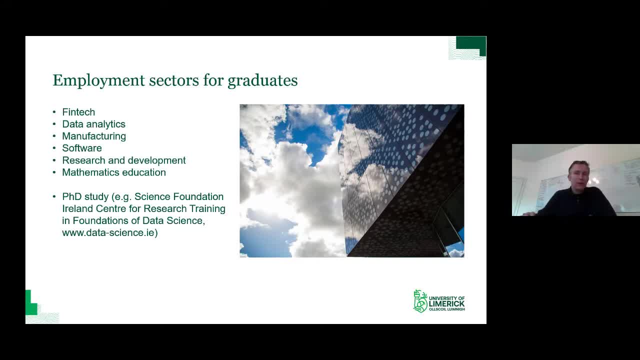 finally, the this masters is a very good route into PhD study if that's something that you're interested in. I'm also the director of the Science Foundation Ireland CRT Centre for Research Training in Foundations of Data Science, which is a collaborative effort led by UL to train. 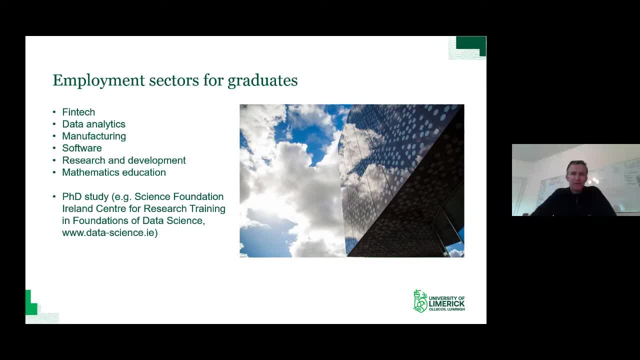 over 130 PhD students in the foundations of data science. data science you've no doubt heard a lot about. people don't always appreciate that mathematical modeling and applied mathematics are one of the foundations of data science, along with statistics and machine learning- those three areas of math. statistics- 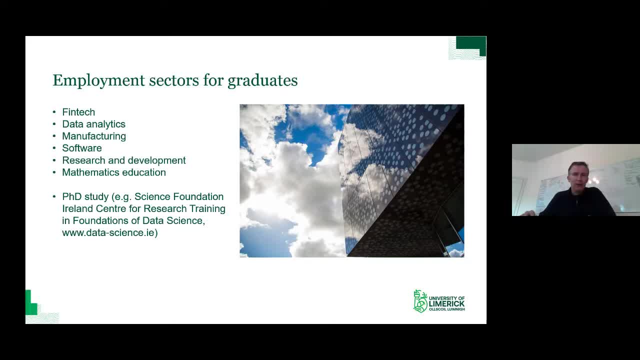 and machine learning are what we call the foundation aspects of data science, and we've gotten large funding and a large number of industry partners who are looking at PhD graduates over the next three to four years. we've already taken in 20 PhD students into UL and we're 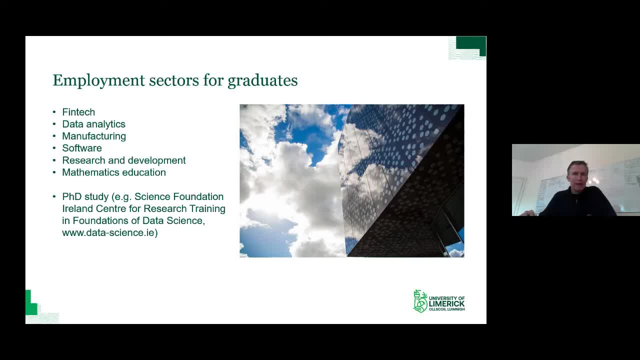 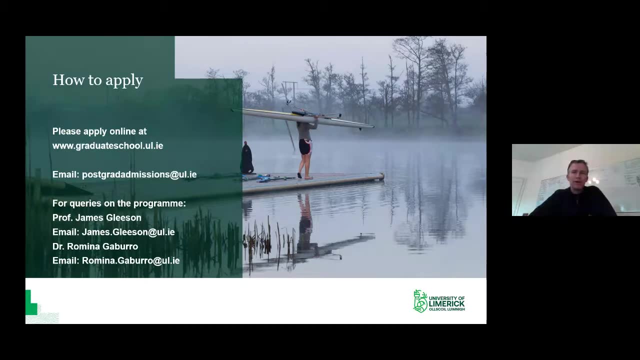 looking to take in more this year and next year in this area and again, we're looking to this masters program as being one of the feeder areas for that. so I'll finish with just leaving you this slide, I guess, on the screen, of how to apply and if you'd like to go ahead, 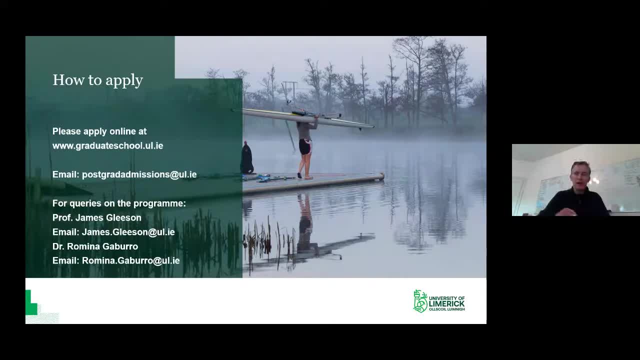 and I'll take a look now at the questions and if you'd like to go ahead and stick any further questions you might have into the chat, I'd be very happy to get to them. I'll read them out one by one and get to them that way. 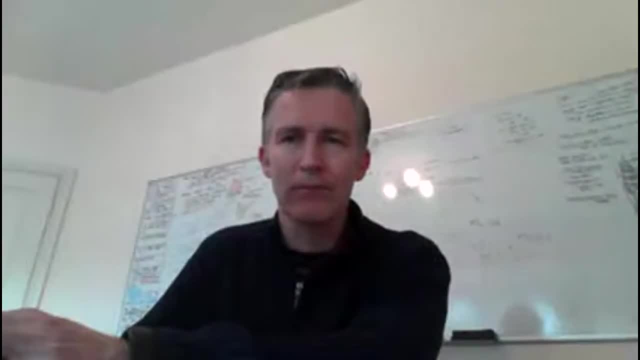 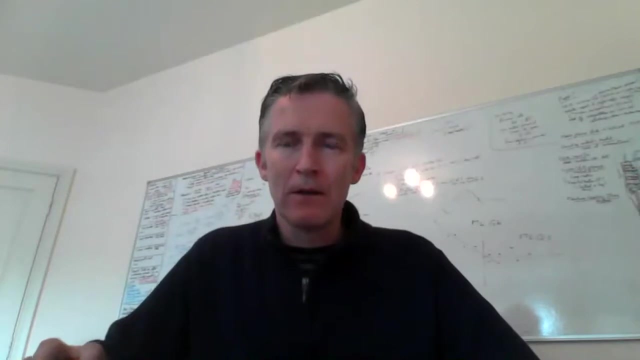 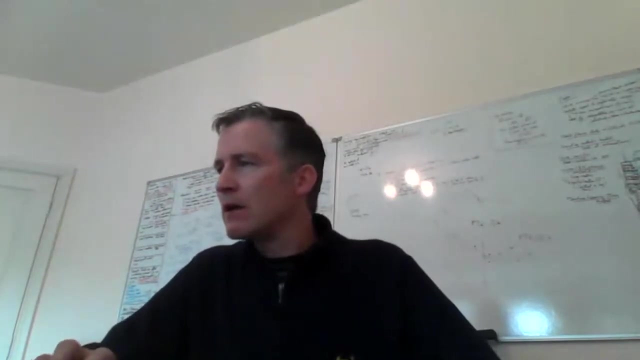 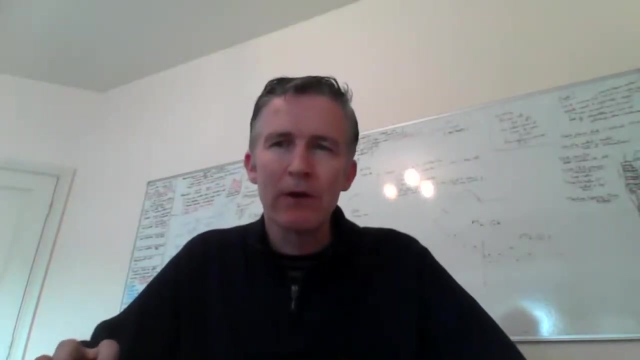 okay, so hopefully you're still seeing me on the screen and I'm going to have a look over here to my side. okay, I don't see any questions at this point, so I'm going to go ahead and see if, at this point, anyone else got any questions there. 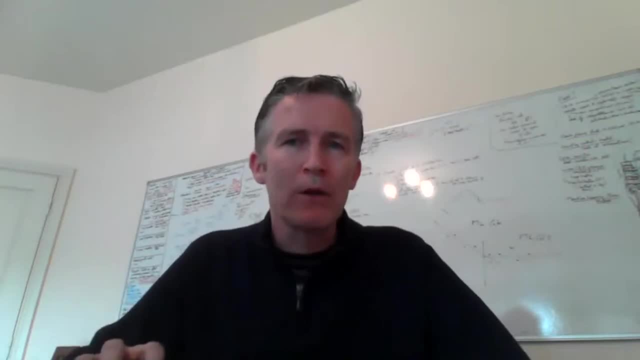 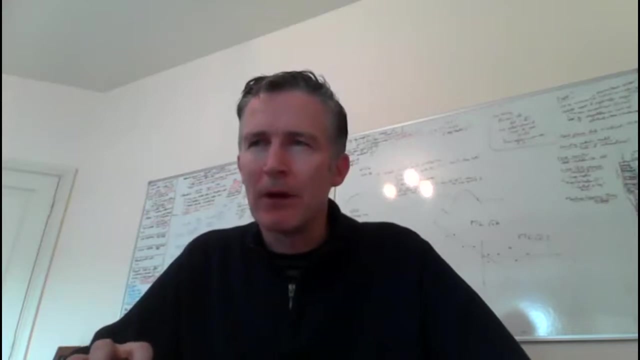 live, or Bernie or Eileen, if anything that's propped up along the way. so no, I'm not seeing questions in my meeting chat here. am I looking in the wrong place? oh sorry, questions answers looking in the wrong place, my bad. so I have a question. 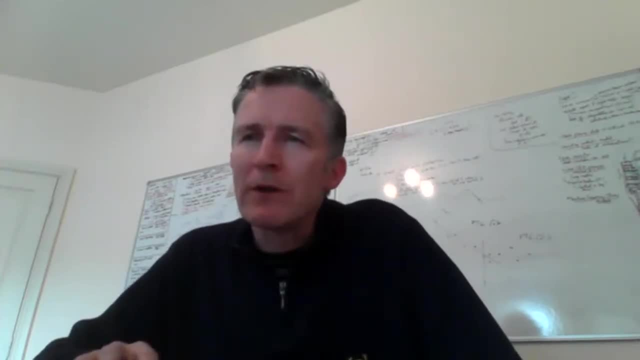 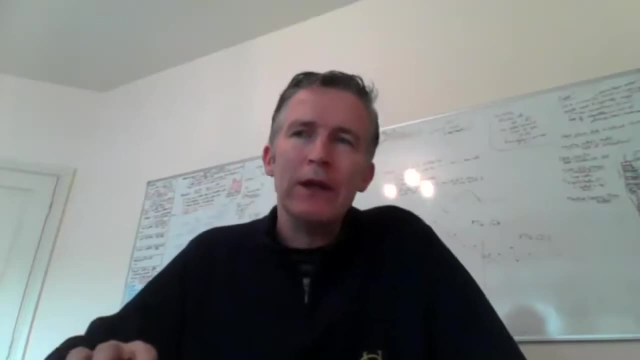 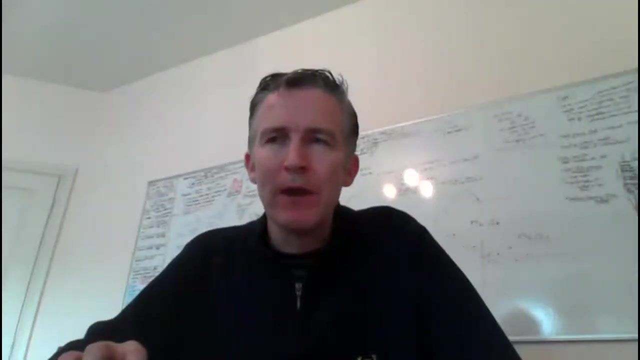 here from Mark. thanks, Mark. do modules such as time series analysis mirror those that make up undergraduate programs like LM058? yes, so, Mark, the elective modules like time series analysis are shared with the final year undergrad courses of the same name, so if you've taken those before, I'm guessing if you. 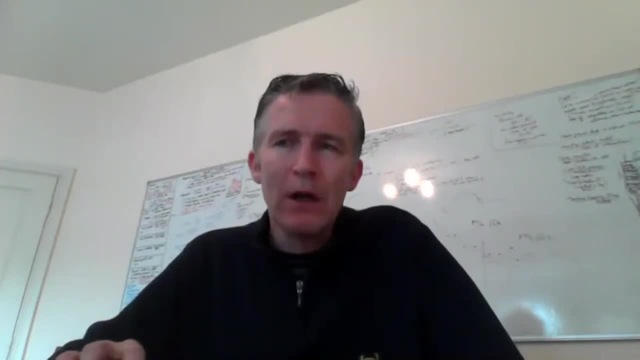 know the course code you maybe have. you've taken those before the. you wouldn't take them again because they're closely aligned and in fact that's true for all entrance to the course. that if they take, if they've seen modules in the past before, in their previous undergrad- 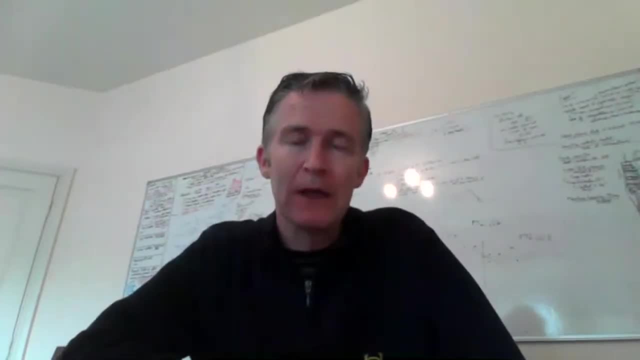 programs. we ask them, we tell them for their own sake not to take those again but to look at other options, obviously to broaden their experience and to think about other directions they could use, although of course you would expect to be able to use that expertise in the master's dissertation, if that's something that's useful. 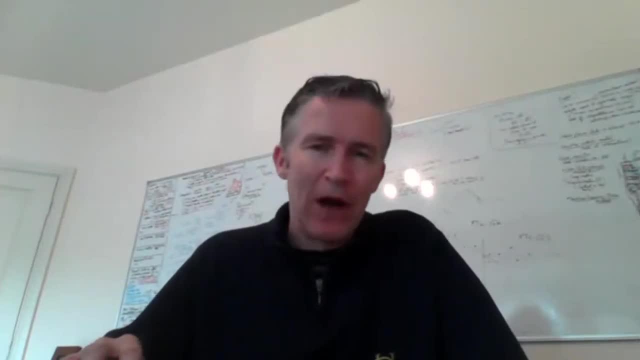 um, having said that, if you haven't taken time series analysis before- not that specific module- the assessment of those modules is different from master's students and for undergraduate students, so in that sense it's not identical. but the course content would be sufficiently similar that if you've seen that, if you've done that course in undergrad, you certainly 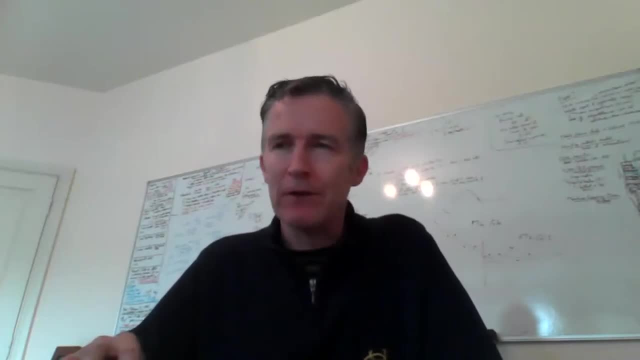 shouldn't take it again. so I hope that answers your question. feel free to fire something into the chat there if anything else pops up. okay, so, um, are there any other questions? that's all I'm seeing. is that question there from Mark on the live events Q&A. 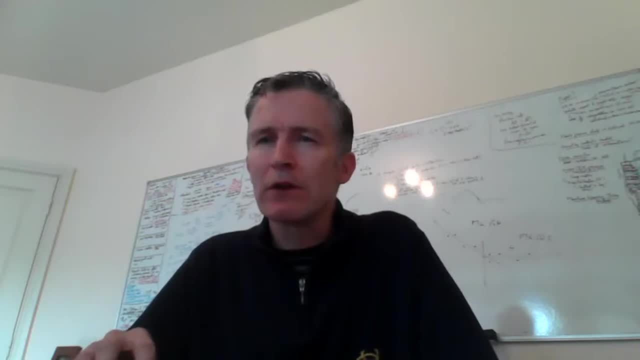 just checking this side conversation, that looks okay. okay, so I think we're done again. if there are further questions, um, or if anything else pops up, very happy to take a question by email. my email is jamesgleeson at ulie. um, and thanks those of you who listened.